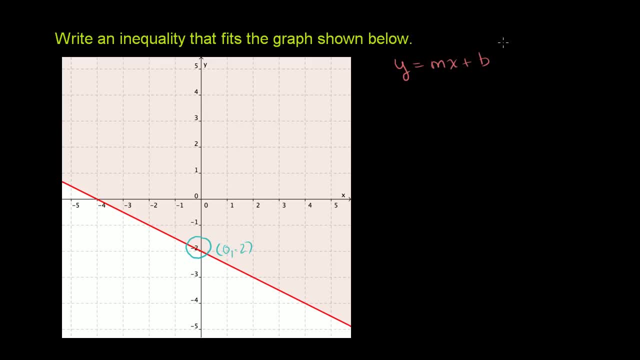 slope-intercept form we figured out, b is equal to negative 2.. So that is negative 2, right there. And let's think about its slope. If we move 2 in the x-direction, if delta x is equal to 2, if our change in x is positive 2, what is our? 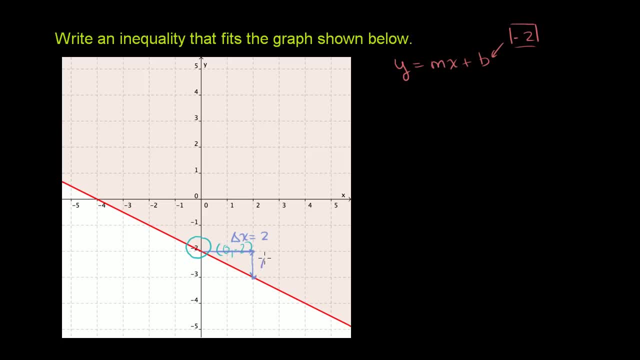 change in y. Our change in y is equal to negative 1.. Slope, or this m, is equal to change in y over change in x, which is equal to, in this case, negative 1 over 2, or negative 1 half. 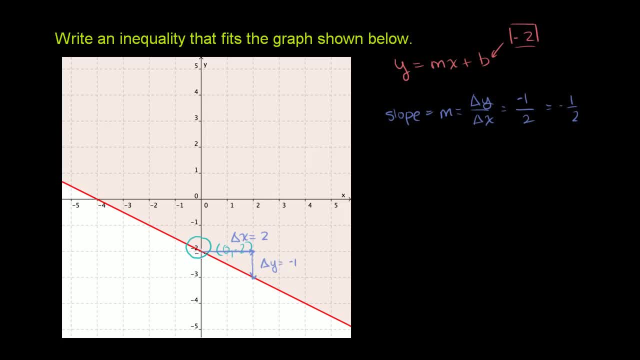 And just to reinforce, and you could have done this anywhere. you could have said: hey, what happens if I go back 4 in x? So if I went back 4, if delta x was negative 4, if delta x is. 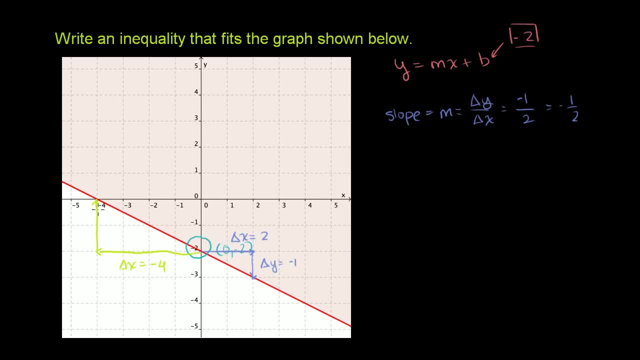 equal to negative 4, then delta y is equal to positive 2.. Delta y would be equal to positive 2.. And once again, delta y over delta x would be positive 2 over negative 4, which is also negative 1 half. 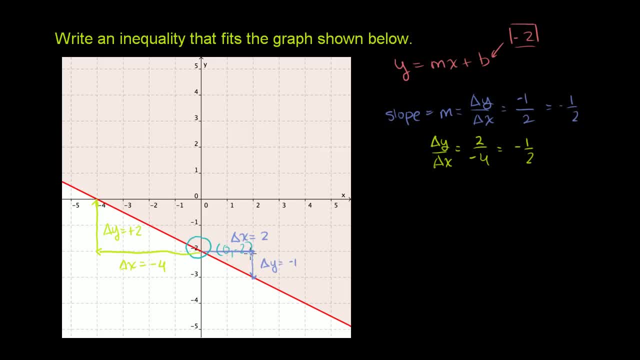 I just want to reinforce that. It's not dependent on how far I move along in x or whether I go forward or backward. It's not dependent on how far I move along in x or whether I go forward or backward. You're always going to get, or you should always get, the. 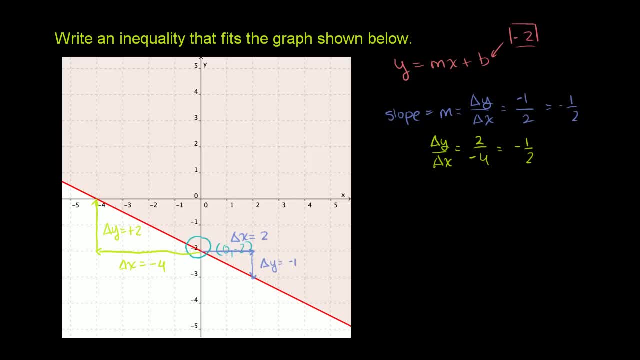 same slope, It's negative 1 half. So the equation of that line is: y is equal to the slope negative 1 half, x plus the y-intercept minus 2.. That's the equation of this line. right there, Now this inequality includes that line. 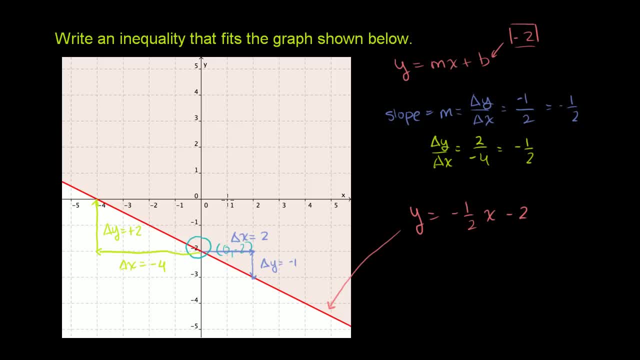 and everything above it. For any x value, let's say x is equal to 1.. This line will tell us: well, let's take this point, so we get to an integer. Let's say that x is equal to 2.. 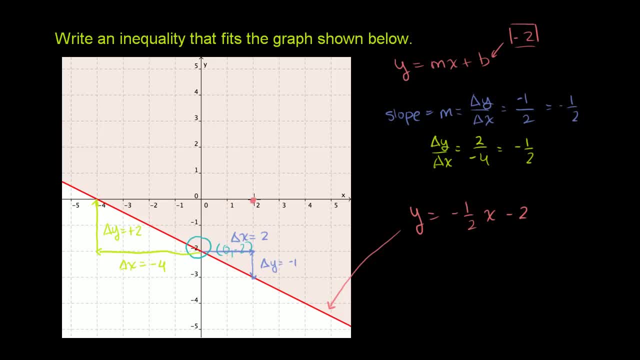 Let me get rid of that. 1. Let's say x is equal to 2. When x is equal to 2, this value is going to give us negative 1 half times 2, which is negative 1, minus 2.. 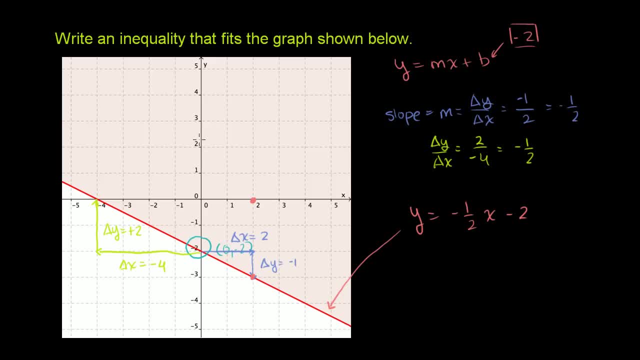 It's going to give us negative 3.. But this inequality isn't just: y is equal to negative 3.. y would be negative 3, or all of the values greater than negative 3.. And I know that because they shaded in this.